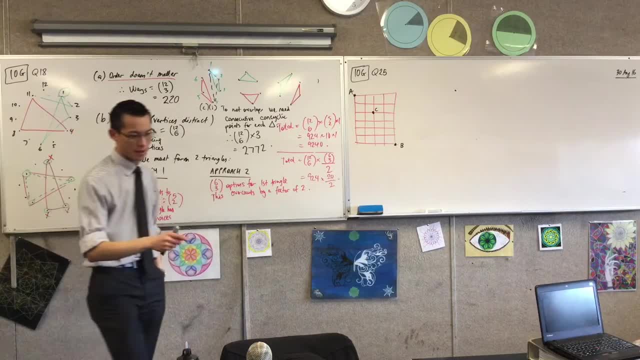 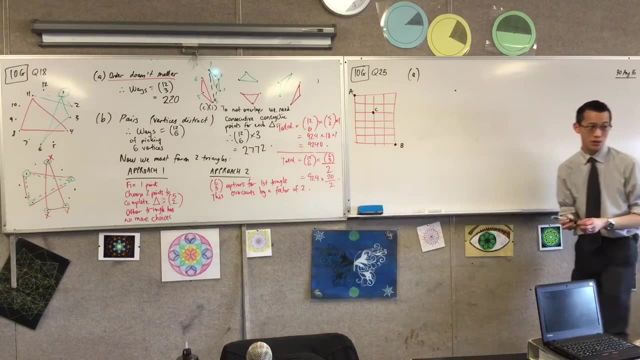 That was a clue. by the way, That was a clue, So let's have a look at this. How many different grids are possible? Now, just like with this making triangles question, I think the lion's share of the thinking in this question is: 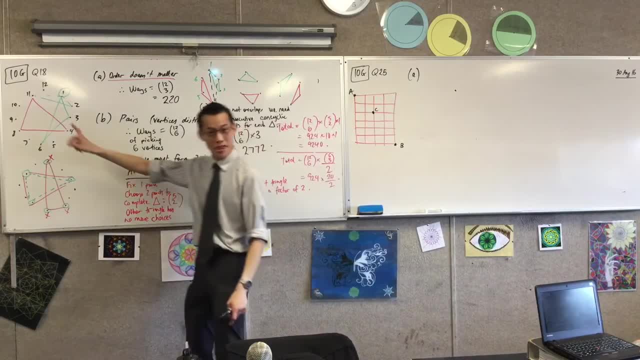 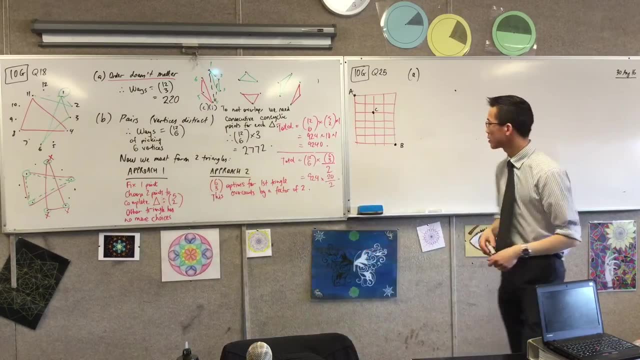 how do I translate this or this into the right language so I can say, oh, it must be this? I think that's the hardest part. So to think about this. remember the rules are: you can only travel to the right or down. 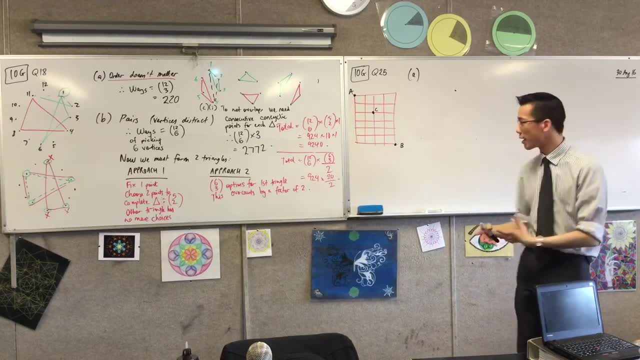 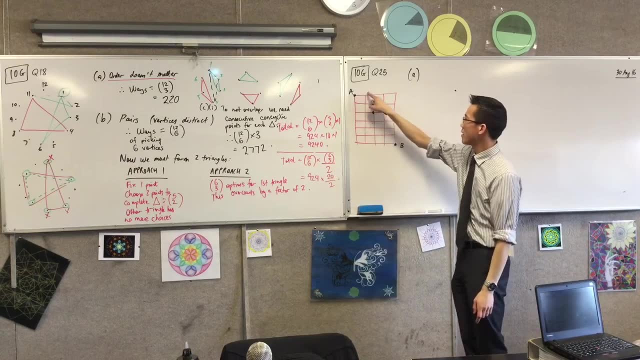 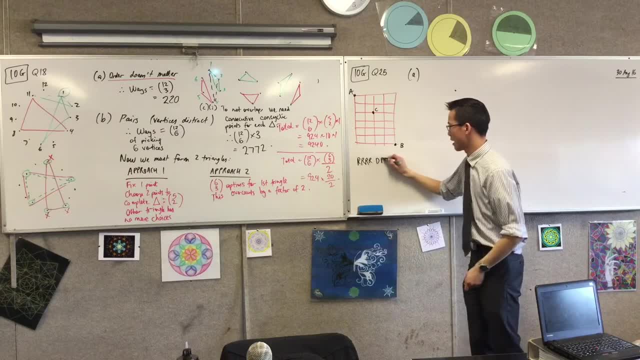 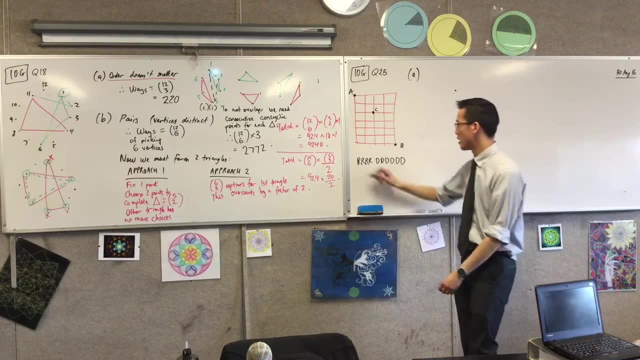 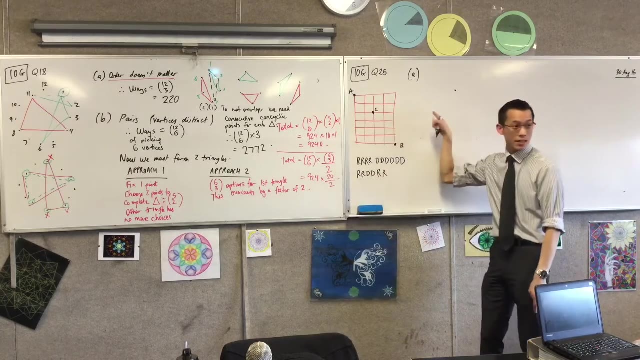 So it would look like this And six of these. This is one successful path through the grid. What would be another one? How about I do a couple of rights, then a couple of down, then a couple more rights. Now, by this time I've hit the edge over here, because I've gone right four times. 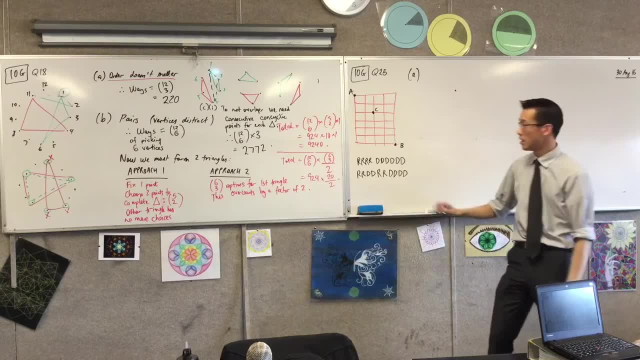 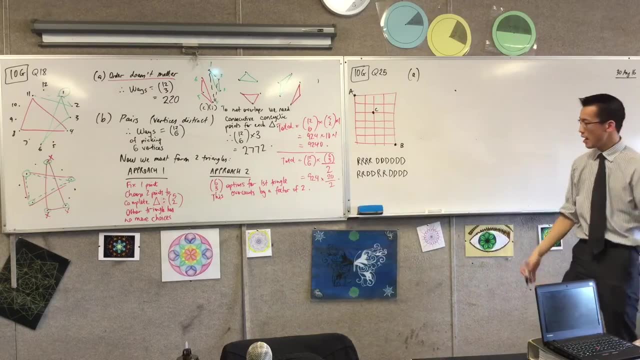 And then I've got four, Four more to go down. Does that make sense? So I can go along here. What's this one going to look like? It's going to go down, across, down, across, all the way down. 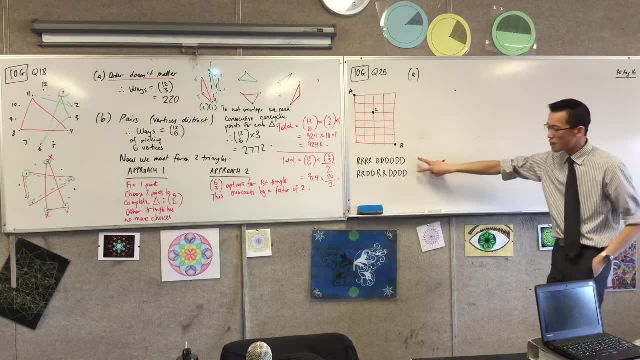 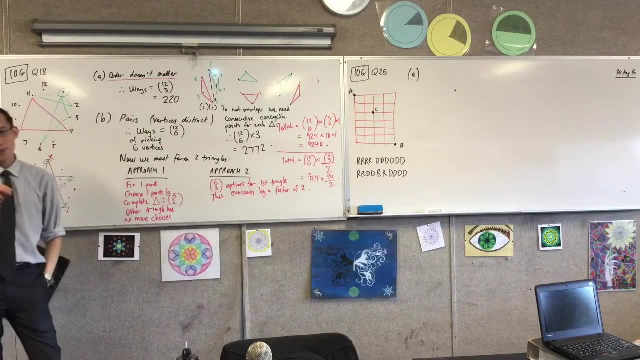 I can keep on going. There's going to be quite a few of them, But hopefully, by writing them in this way, you're starting to click. Okay, what kind of question is this? I have to? is it different to do this versus this? 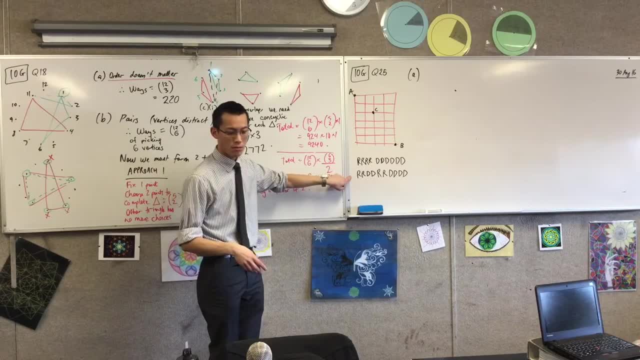 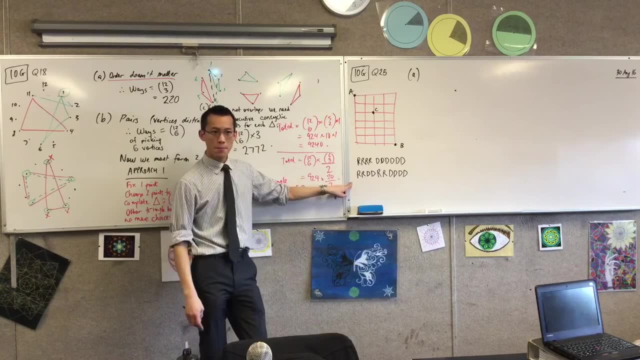 Are these counted as different ways? The answer is yes, They're different routes, Are they? They're different routes. Now, what's the difference between these two? The only difference is order. Okay, so I'm in permutations land. Does that make sense? 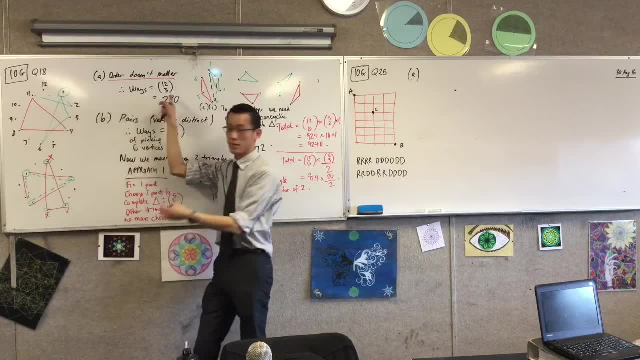 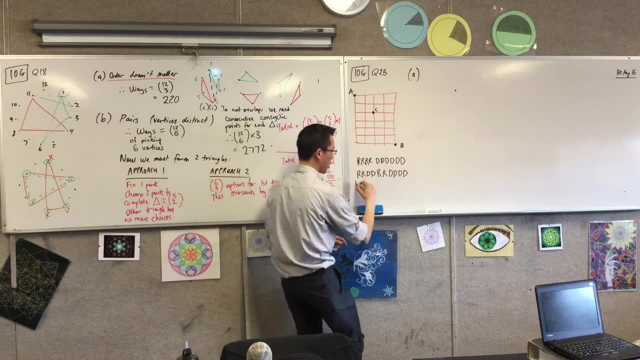 So I had to think carefully like: what kind of question is this? Okay, this is the tool for it. What kind of question is this? It's permutations. Now, also, I want you to know what I've got to do. 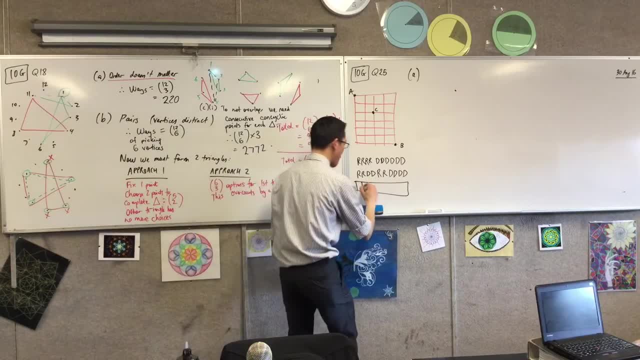 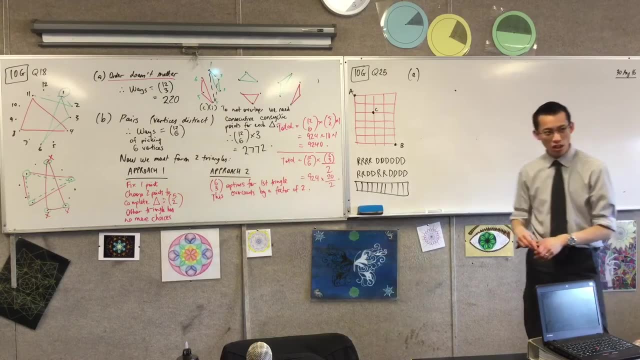 And they gave you this clue in the question: right, I have to make exactly ten moves. Did I do it right? Yes, I did. I have to make exactly ten moves, right. It's not like you've got some moves and you only choose some of them, right. 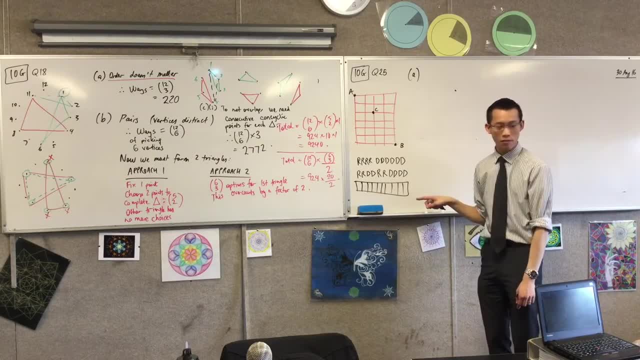 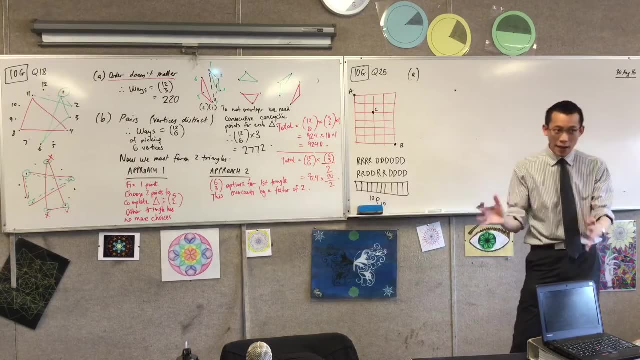 You've got ten moves to do and you've got to fill every single one, right? So this is not just permutations, This is ten p ten, right. You have to pick ten things to fit into those spots And, by the way, that's ten factorial. 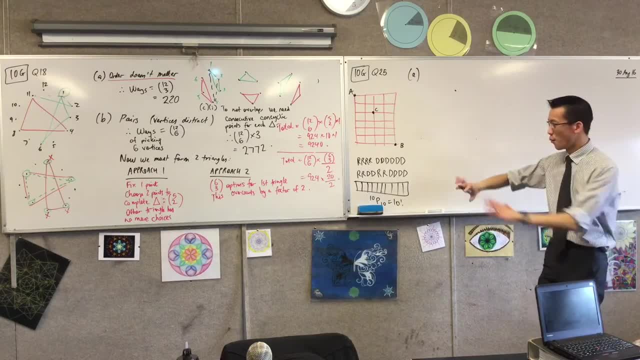 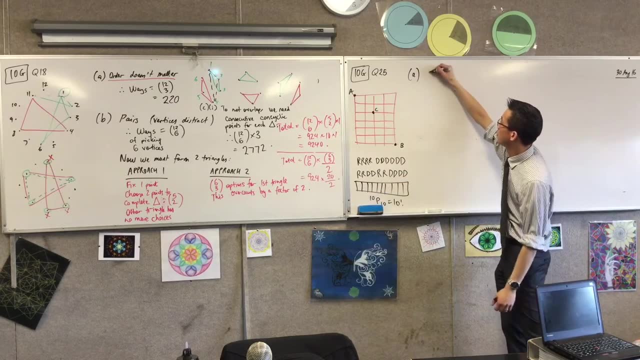 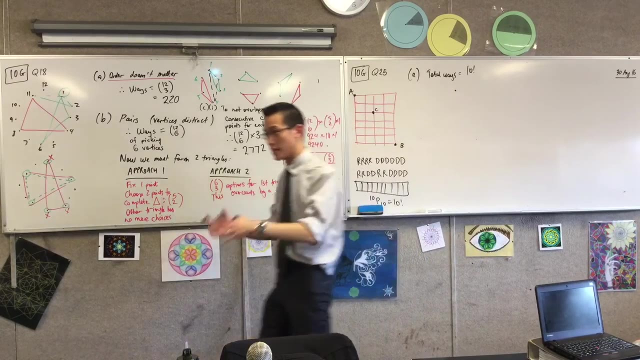 Remember that one. Okay. So working out how many ways to choose a series of ten objects to fit into ten spots. this is my first one: total ways. I have to begin by saying ten factorial right, Ten spots, ten things to put in those spots. 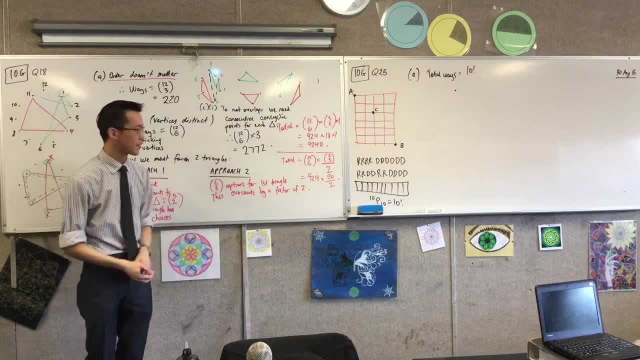 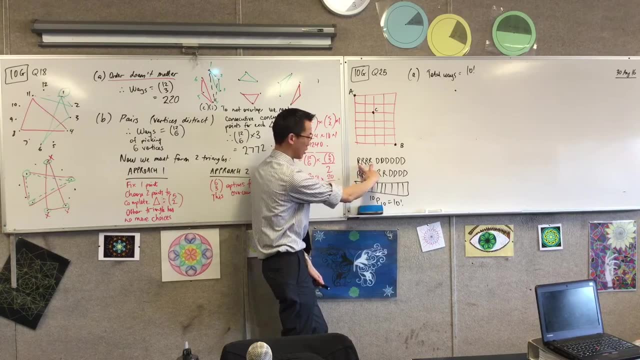 there are ten things to put in the first one, nine things, et cetera. Ah, but of course you're like hold on a second If, for instance, you took these two guys, this right and this right, and switched them. 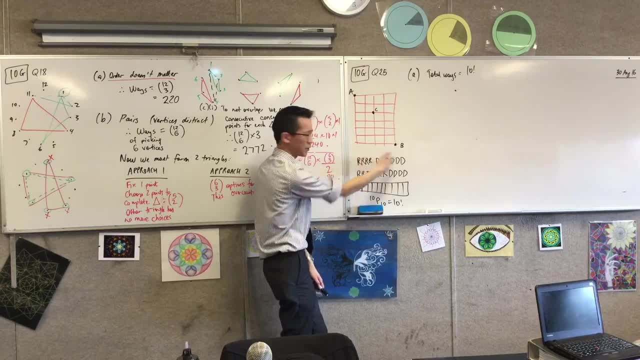 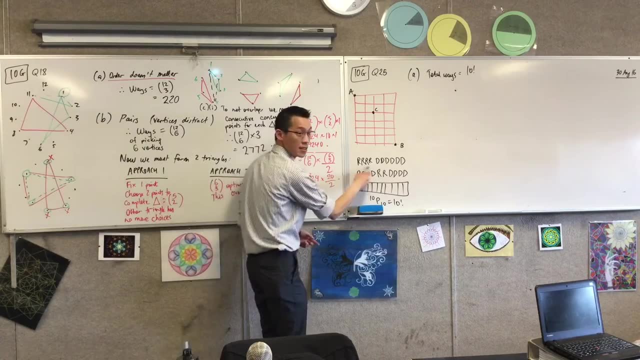 you'd be like: but that's the same, because they're both rights. I can't tell the difference in any of these, right? So I have identical areas. I have identical elements, don't I, Right? So you see these guys. 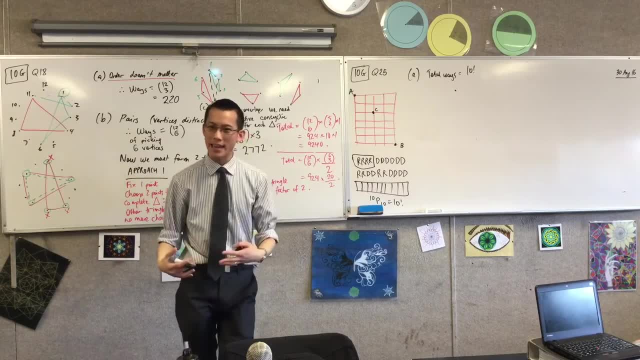 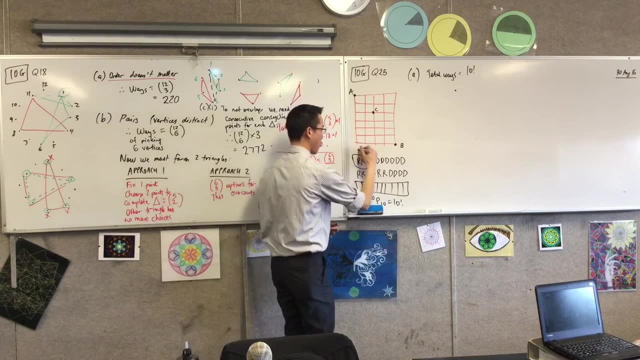 These guys here. How many ways can these turns rearrange themselves? and I won't be able to tell How many ways. Answer: four factorial, So I've overcounted by that factor And then these guys can rearrange themselves too. 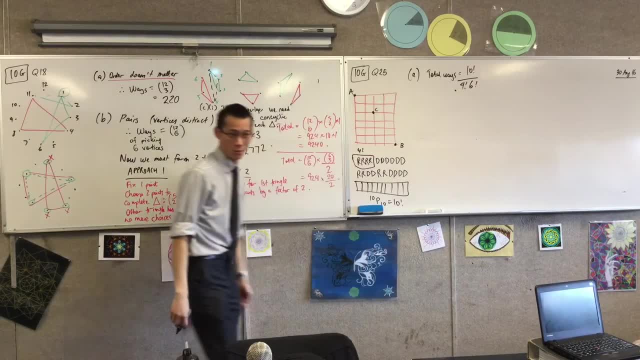 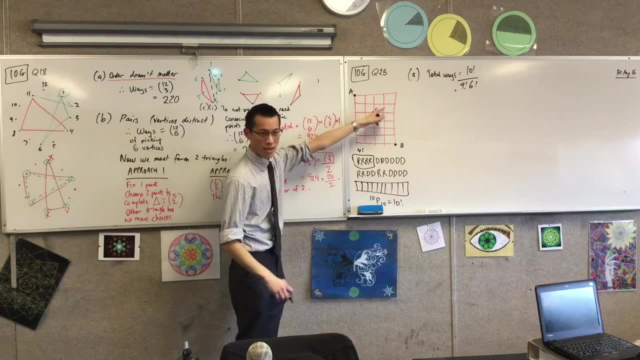 in six factorial ways, So I've overcounted by that as well. Okay, Remember I told you the lion's share of this question is in seeing through this to what is it really asking, Right? How can I phrase this question in a way that renders it? 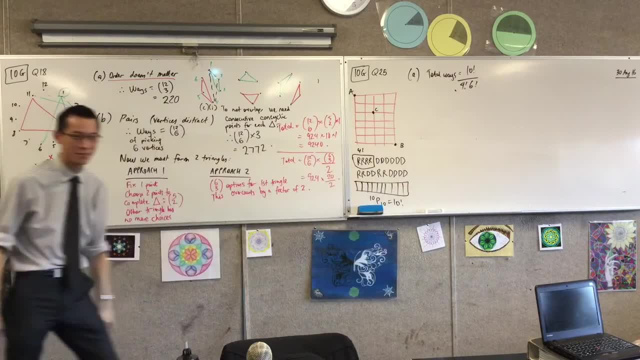 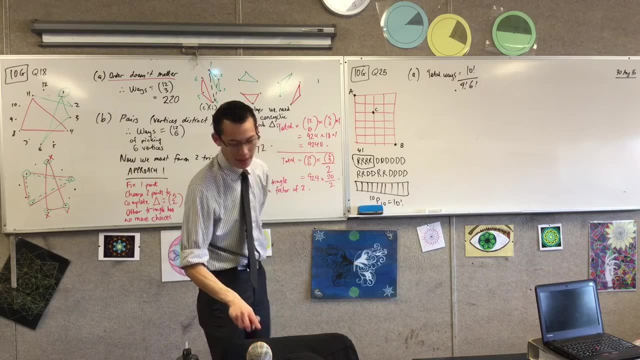 you know, helpless at the mercy of the tools that I have, All right, So now maybe you can walk through and do the rest with me, Right? Part B says how many ways are there from A to B via C. Okay, 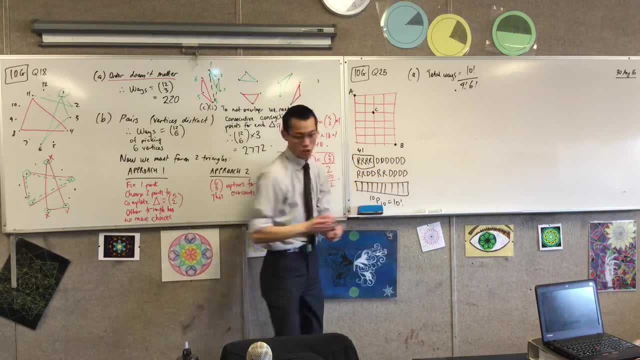 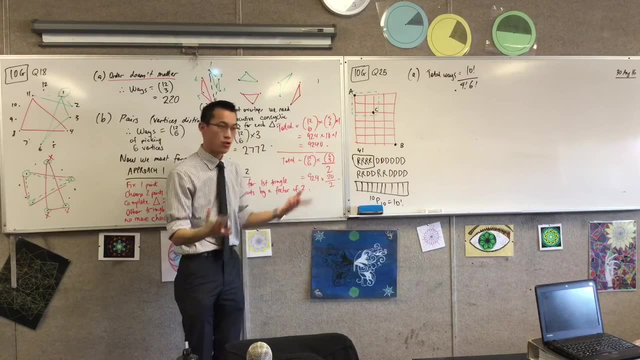 Now, what this is is breaking one journey into two pieces. Right, Firstly, you have to get from A to C. You have to do that Like, otherwise you'll miss C and you won't meet the condition. And then, after you're at C, you've got to get from C to B. 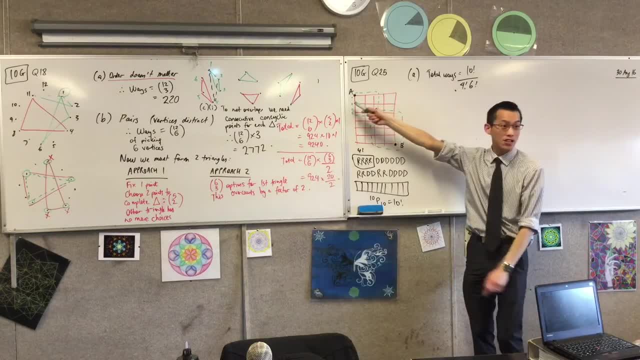 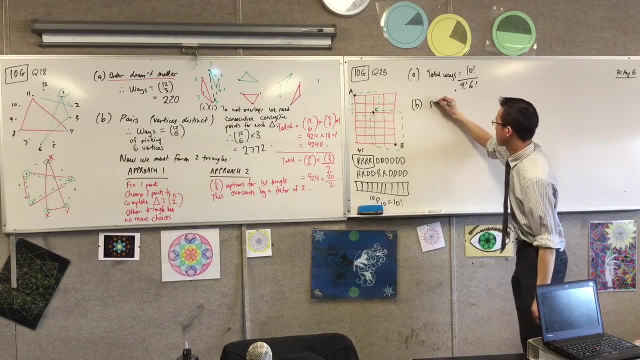 Does that make sense? So I just have to do the first part of the journey, then do the second part of the journey. Okay, Think about it. It's Part B, To get from A to C, From A to C. 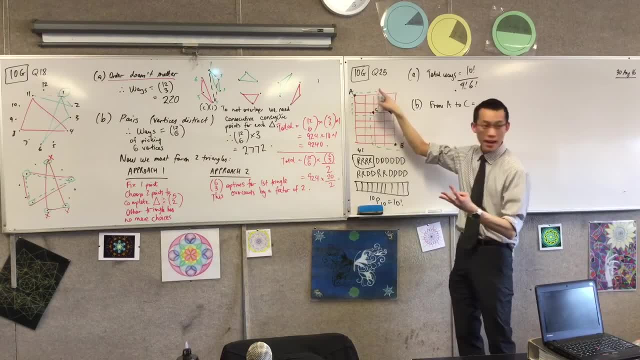 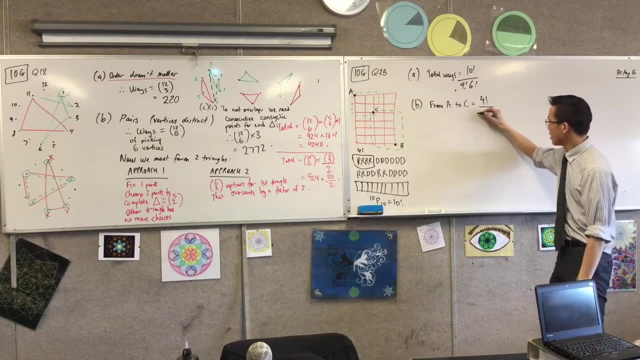 How many turns is it going to take me? Four turns right, Two right and two down, So I've got to fit four moves into four spots, but there are some repeated. There are two rights that can swap and I won't tell. 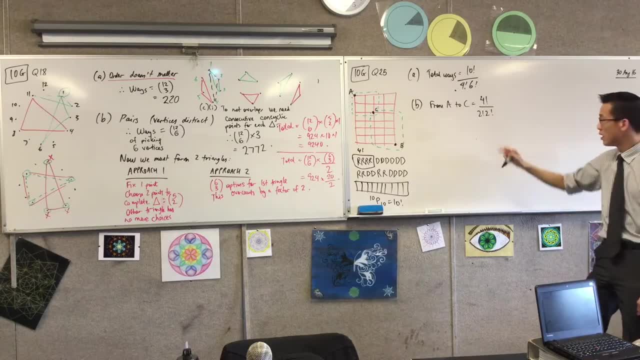 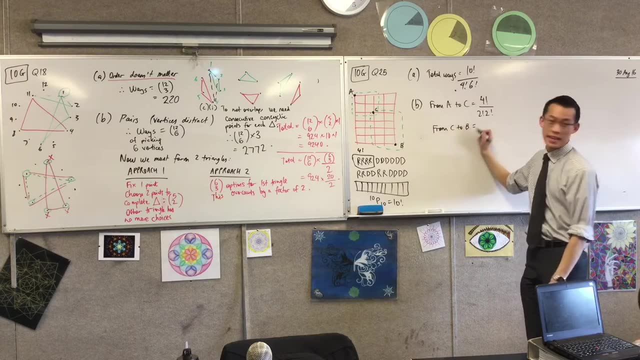 and there are two down that can swap and I can't tell. So this is how to do the first leg of the journey, and then you can tell me how to get from C to B. How many steps, Six, Six steps. 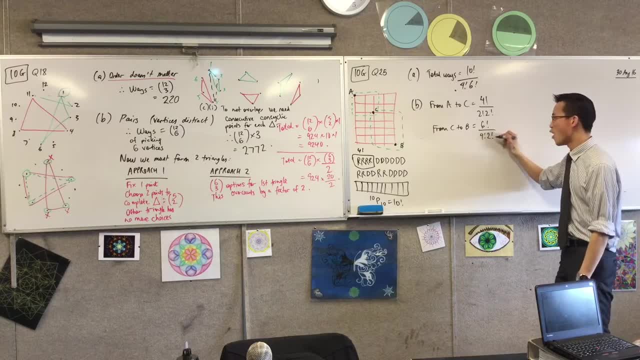 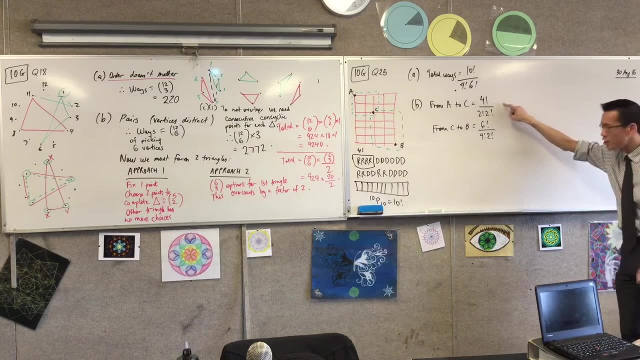 But there's an over-counting factor of etc. Okay, But, but you need to do these And you need to do these, Otherwise, if you don't do both together, you don't get to B. Okay, So you don't add them. 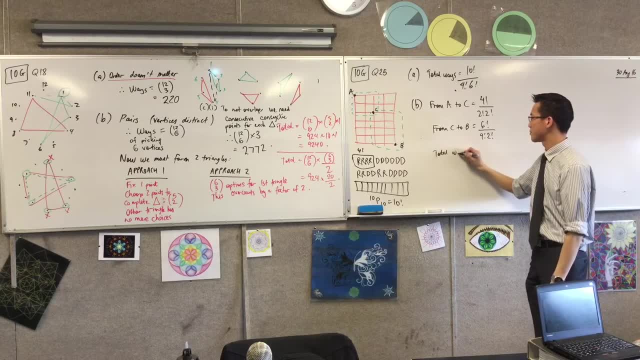 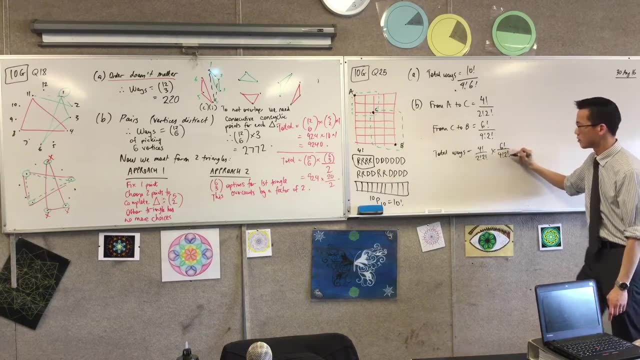 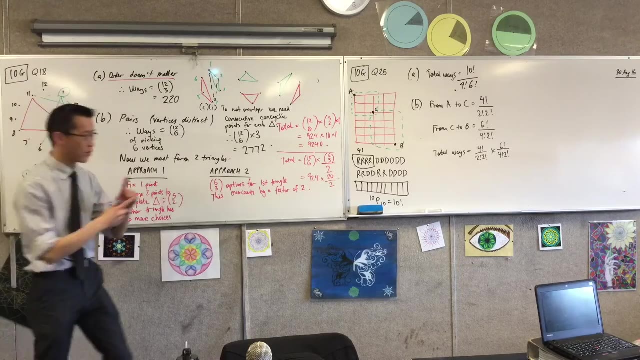 You multiply, So the total ways are this: one by this one. Whatever that number happens to be, I think it's 90, from memory, Six times 15.. Six times 15, which is 90.. Okay, So seeing in here, it's just a small. 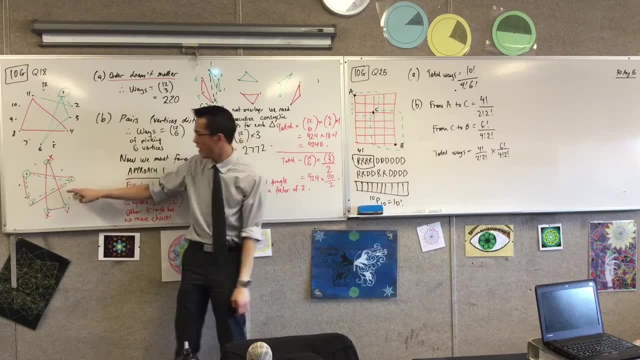 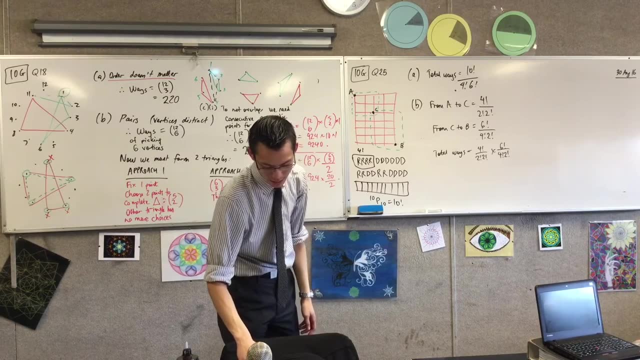 but that's exactly what happened here. Did you notice that Right? So in the question there are smaller versions of the original question. Okay, Part C. Part C. They say: okay, this top line is off limits, Right. 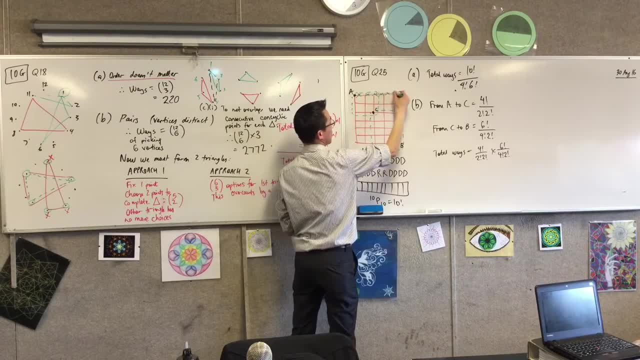 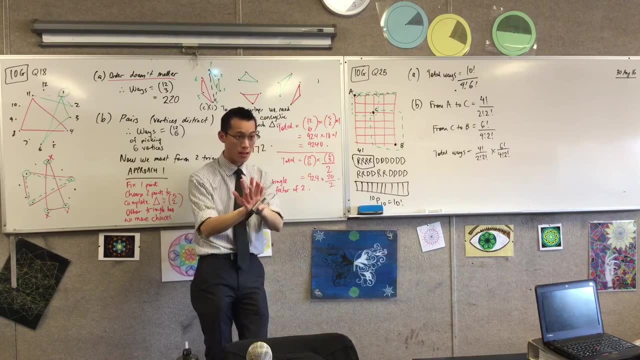 They're like no go, No go. Can't do that Right. So therefore, from A. now, how many options do I have? from A? There's only one way I can go. Got to get to here? Let's call this spot. I don't know. let's call it X. 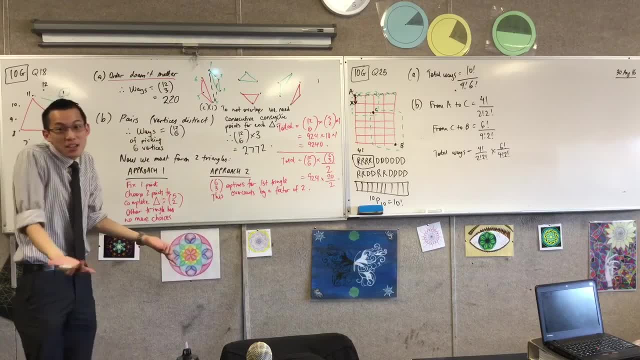 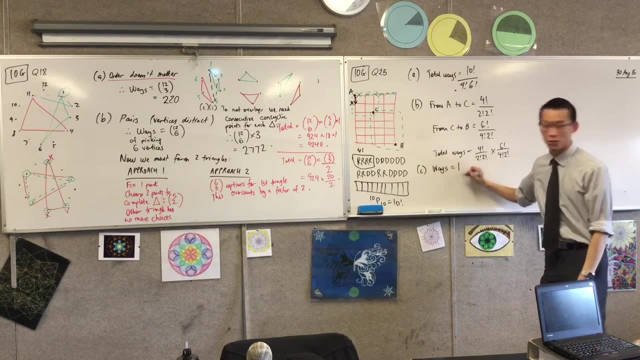 Okay, And then you've got to get from X to B. Are there any restrictions on how you get from X to B? Nope, Nope. So therefore part C: the total ways are: firstly one: There's only one way to get off. A. 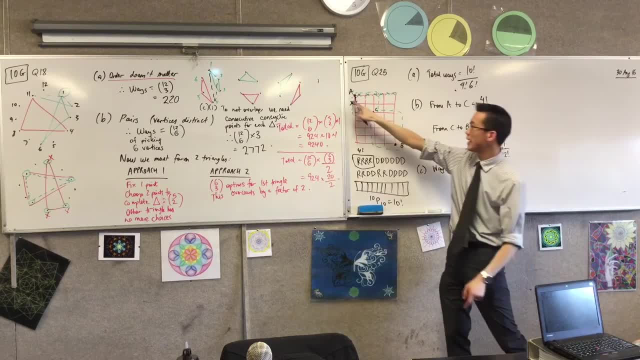 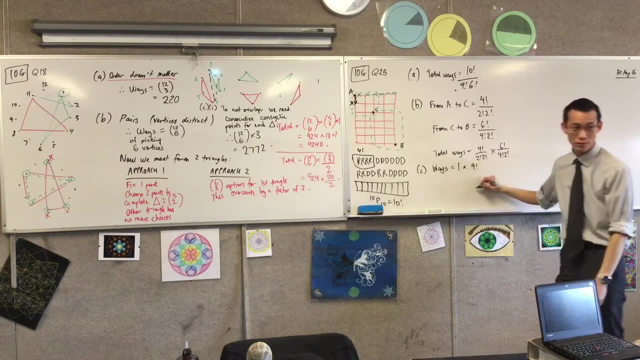 I'm just going to write one And then I've got to go from here to here. How many ways from X to B, How many- sorry, I should say how many moves from X to B. There's nine factorial nine moves, right. 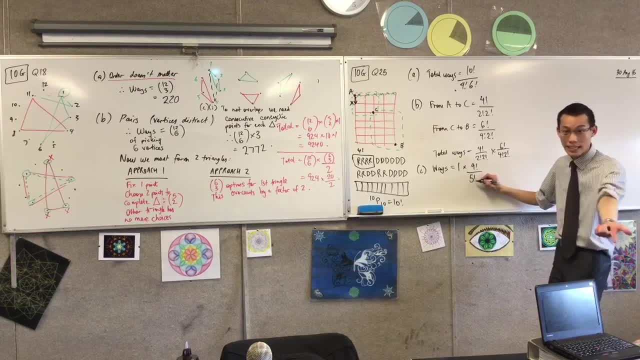 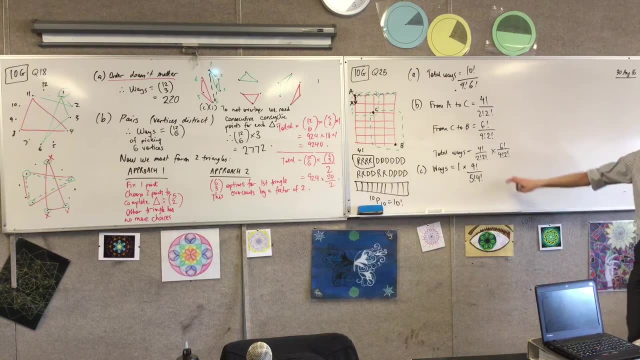 But yes, that's right. I have to do five steps down that are all identical, and I have to do four steps to the right that are all identical. okay, Isn't that at the same? And C5 and 4,, those are all identical. 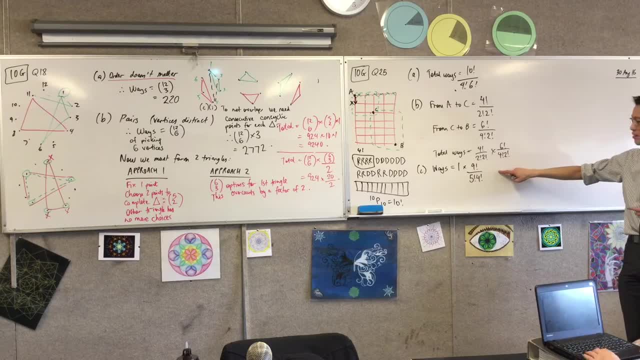 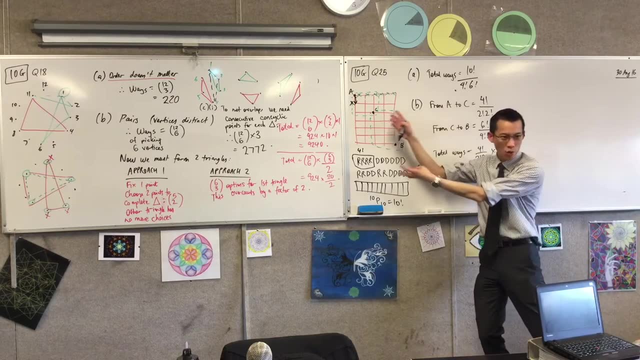 Yes, Yes it is, Yes it is, But yeah, so in some ways coincidentally. okay, Because these two numbers here come from the fact that I've got identical objects, not because there's this factorial and this minus that factorial. 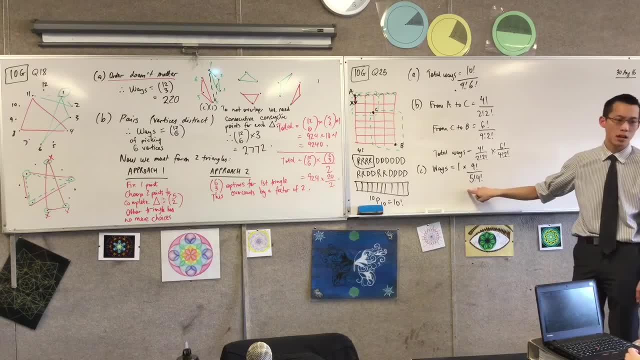 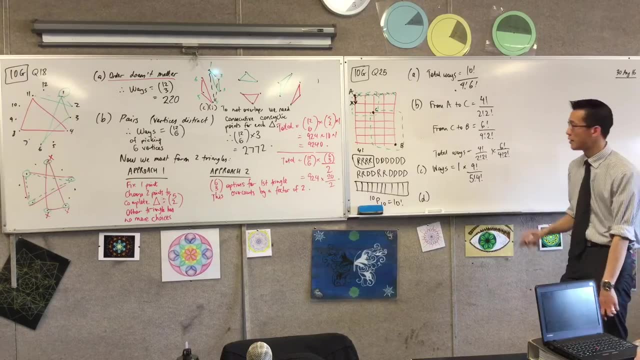 They didn't have to be like exactly matching and identical, okay, But yes, this happens to be nine C5, okay, Last one, last one. So that was avoiding the top line. Now they're saying, actually, you know what? 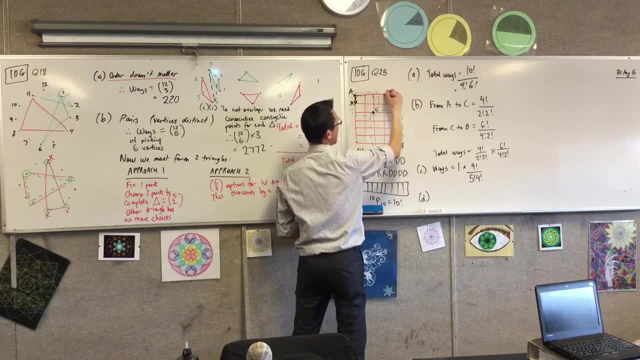 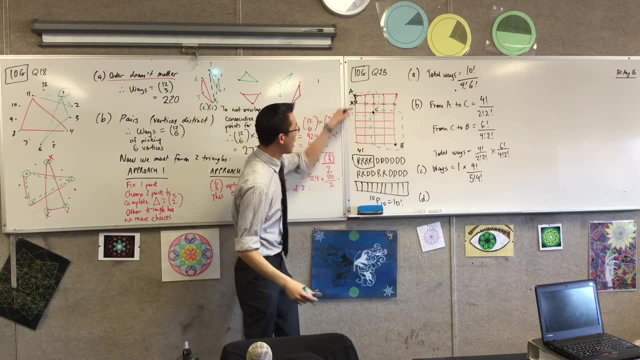 Top line's. okay, Let's put this guy back. But now it's the second line, that's a dud. okay, Now cross, cross, cross, cross cross. So I can't travel to the right here. I can go through it. 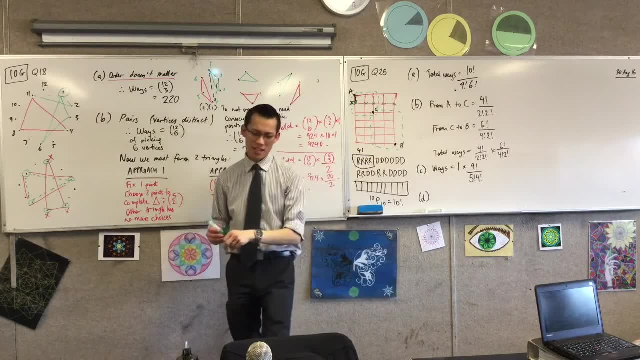 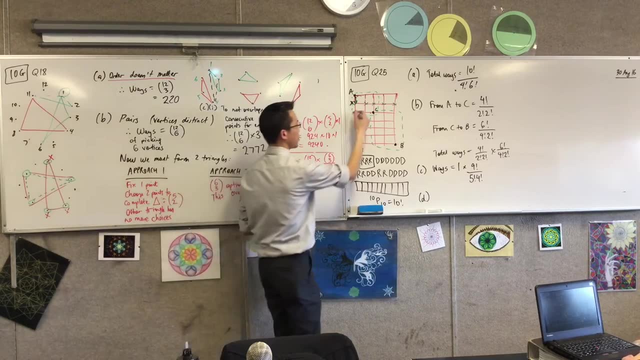 I can go through it, but I can't travel on it. okay, Now this becomes a little bit tricky, but not that much, not that much. I'm going to try and break this down to size. okay, So I've got these. 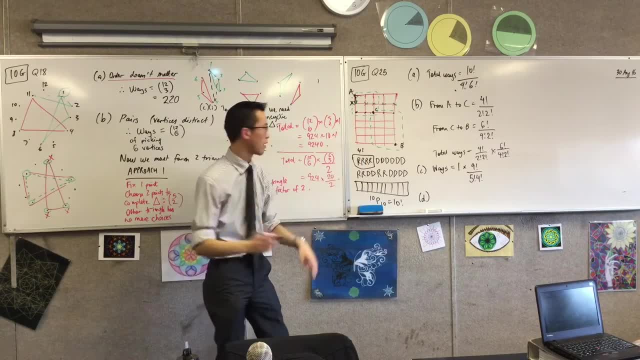 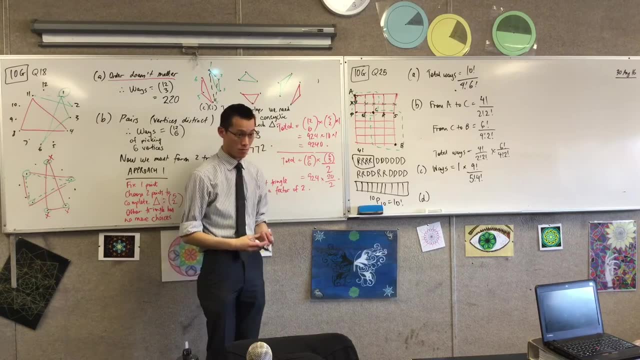 I've got these points under here that I have to get to one of them, right, So I'm going to give them names: P, Q, R and S, okay, And you can see how many ways are there from A to P. 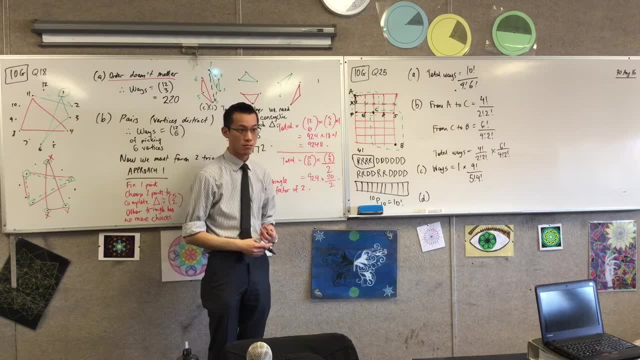 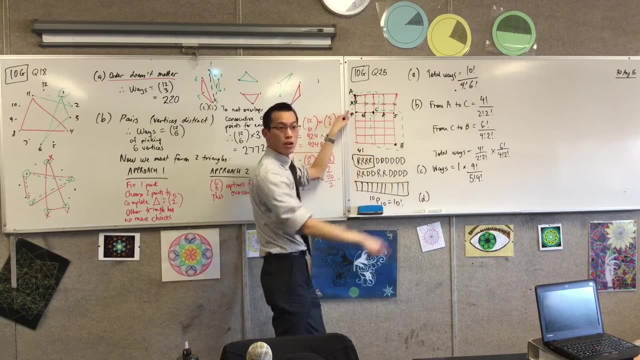 How many ways from A to P? Well, one, There's only one way, right? So I've got to get from A to P, and then I have to do this journey, on which there are no restrictions, right? So this is. oh, I'm going to need more space. 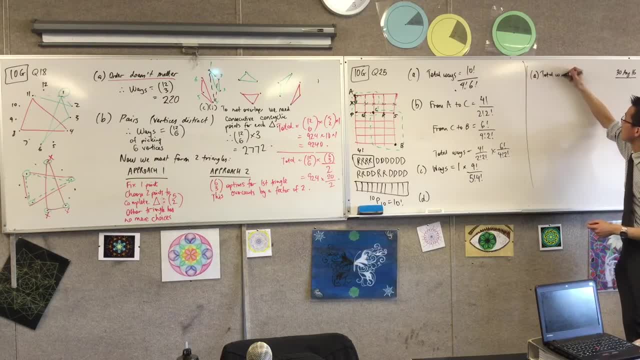 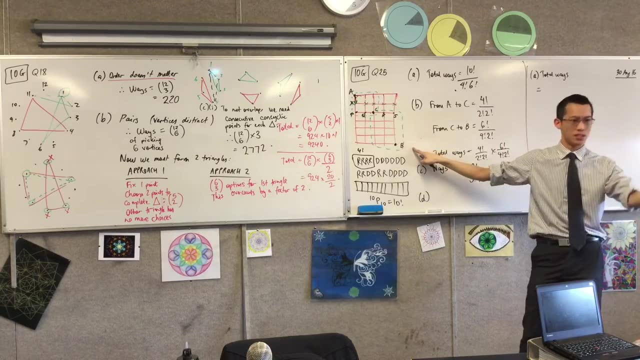 What I'm going to do is I'm going to say the total ways I can get from A to P. that's okay, but then I've got to get from P to B, and there's lots and lots of different ways I can do that. 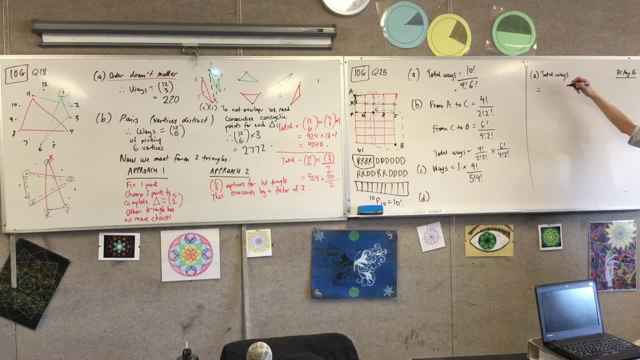 Does that make sense? So therefore, I'm going to say that's going to be equal to: let's see here, P to B, How many steps, how many moves from P to B. I think it's eight, right? So that's eight factorial. on. 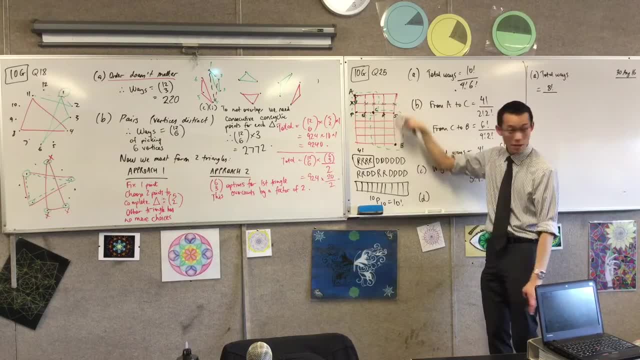 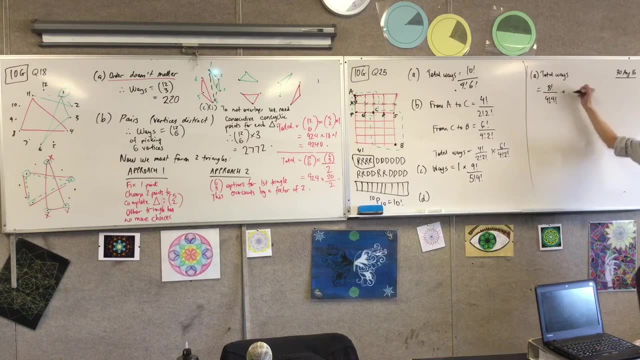 there's four that are the same here, that are identical, and four that are the same here, that are identical, Four factorial, four factorial. Is that okay? Yeah, okay, But that's not the only way to get there. and I'm adding, I'm adding. 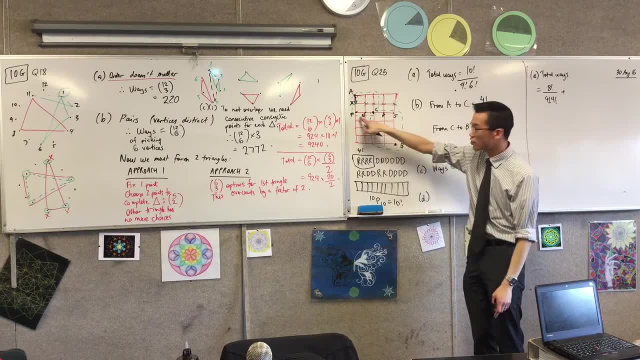 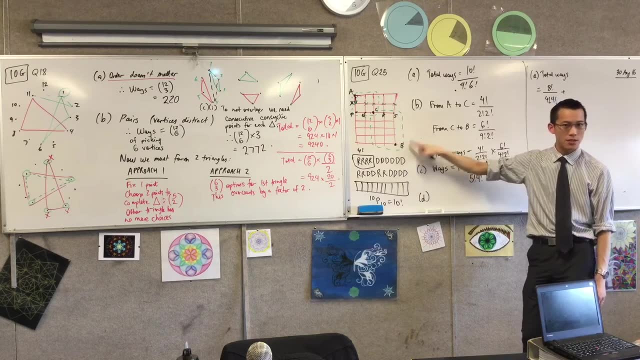 because I'm now thinking about going from somewhere else. okay, So I want to treat Q as my launching pad. now, right, So I'm going to get to Q, and then I'm going to think, well, how do I get from Q to B? 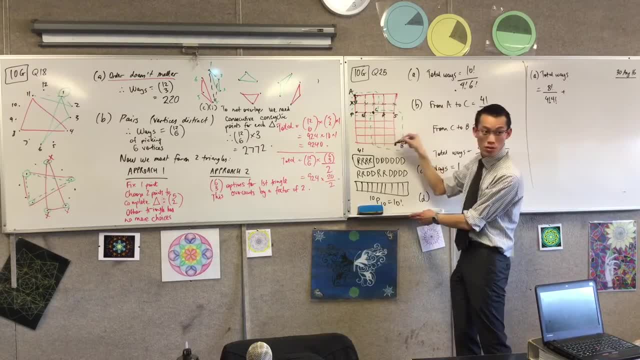 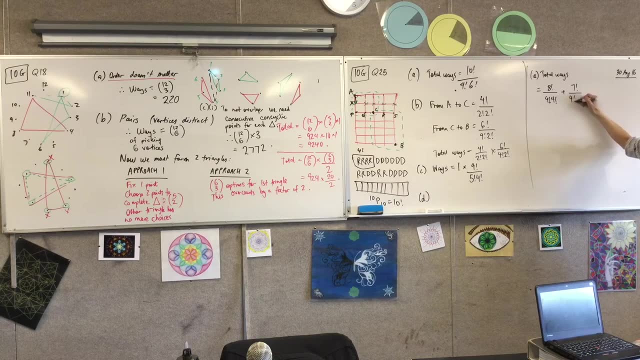 From Q to B. Well, it takes me seven moves to do it. seven factorial, right, But some of these moves are identical and I can't tell the difference. Four factorial, three factorial over counted because of the R's and D's that are the same to me, okay. 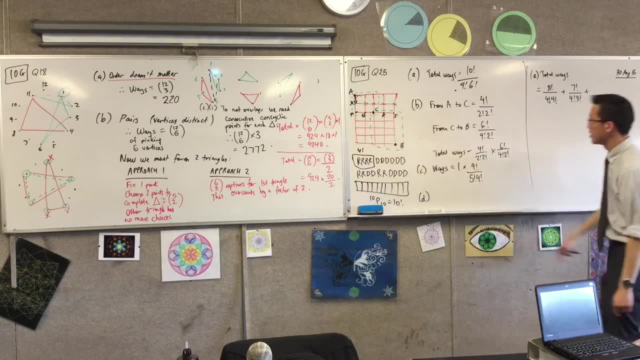 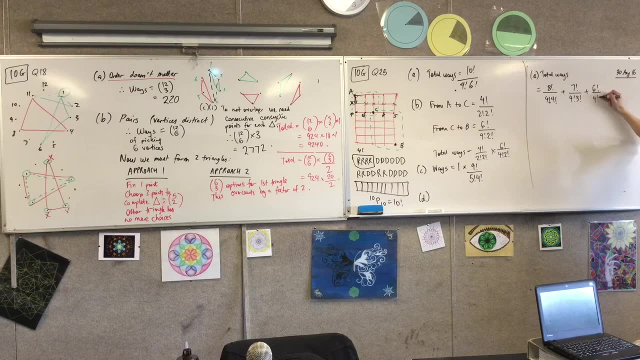 And then I've got C, and then I've got R, and then I've got S. So let's have a look at this. How does the pattern unfold? Let's see six factorial on: Yeah, yeah. Then I've got to go from R, which is this guy. 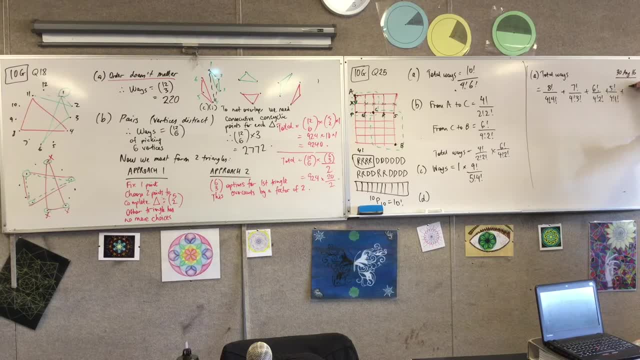 four factorial, one factorial And then, lastly, I've got to go from S. Now think for a second right, Think for a second. I've got four moves to go right, But all four of those look identical to me. 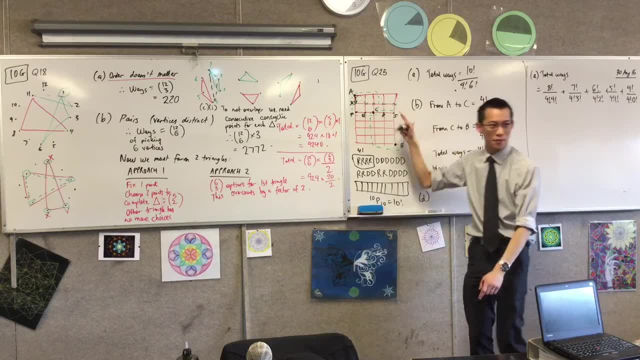 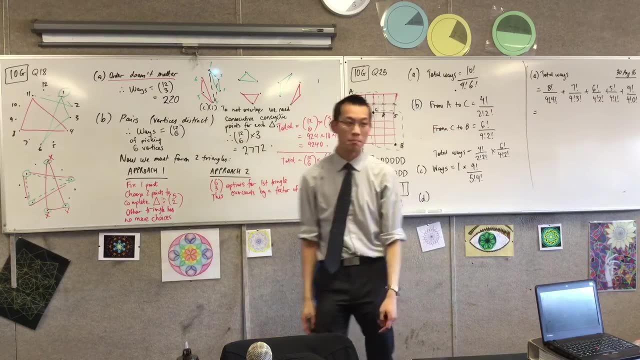 So I've overcounted by all those ways and, of course, because there's only one way from S to B, Does that make sense. So that's why that last guy is just one. So I have no idea what happens when you add those all up. 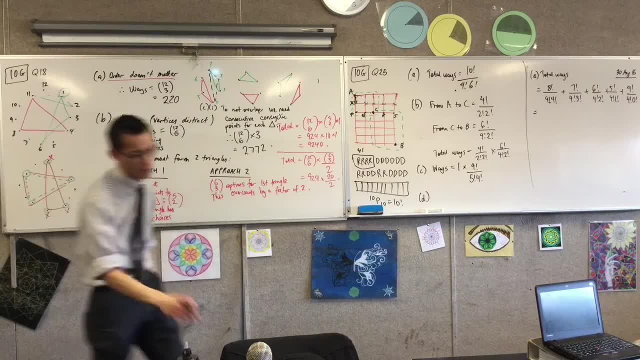 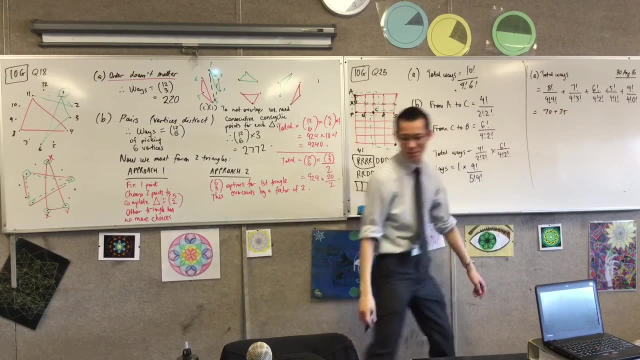 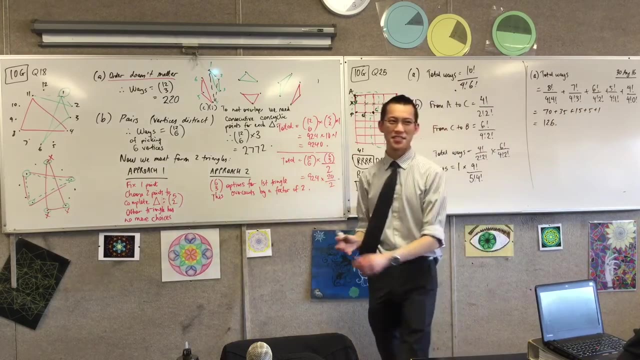 but those are all the cases. okay, Those are all the cases. I've got a number actually. So in this instance, you factor. Yeah, yeah, you can do some factorizing here. I counted them, I got to like 20, and I was like, how, not? 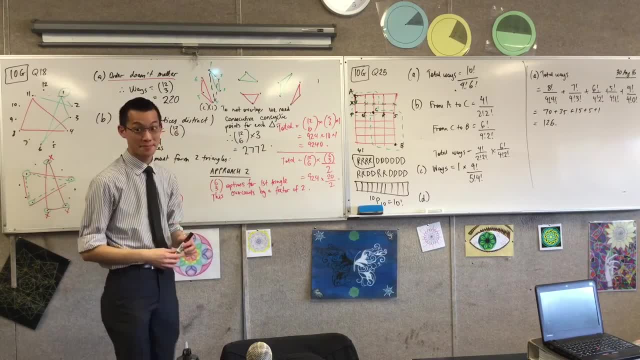 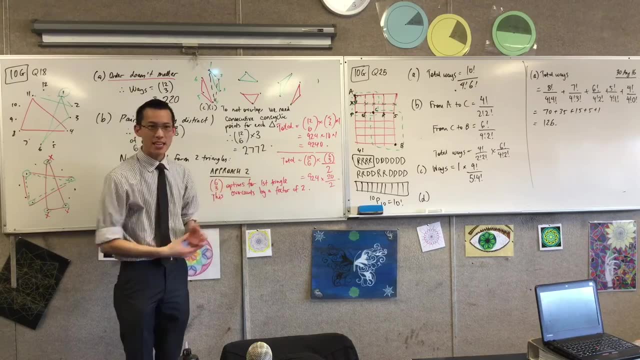 As soon as you wrote the first line, I got it I was like, ah Now, by the way, I'm glad Mark mentioned it- C and D. they have the same answer, C and D- But why is that? 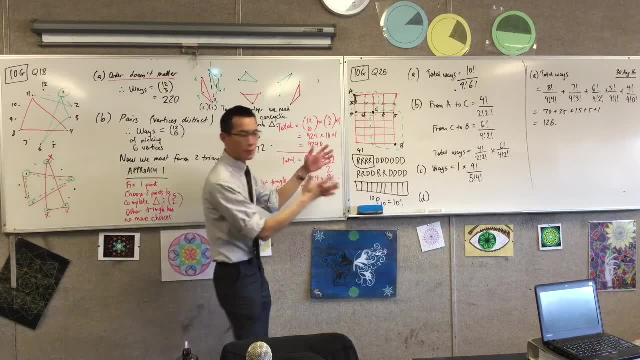 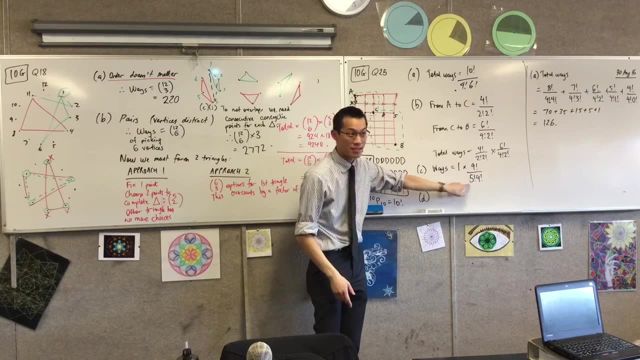 Well, you're both times including one row. That's exactly right. Both times you simply turn this six by four thing into a five by four, And that's why it's the same problem. See that, That's just five by four.